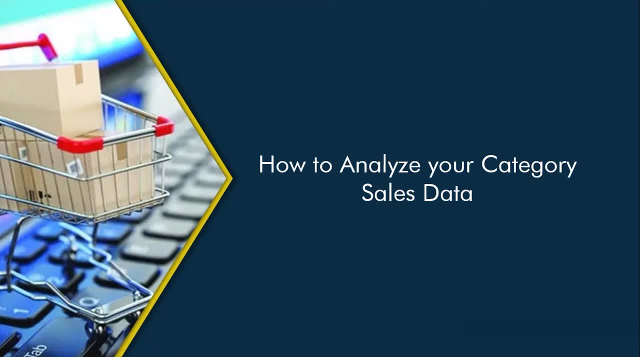 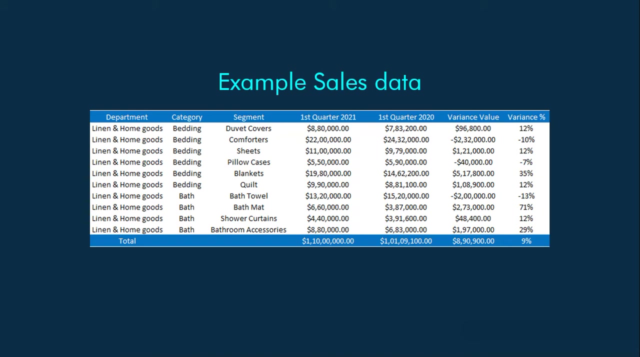 you have to have a clear sales data with the proper analyzation. The more you analyze your category sales data, the more you have a better idea about your customer purchase behavior as well, As well as your assortment. This is a simple sample data. I have taken it just to share in this video. This is just 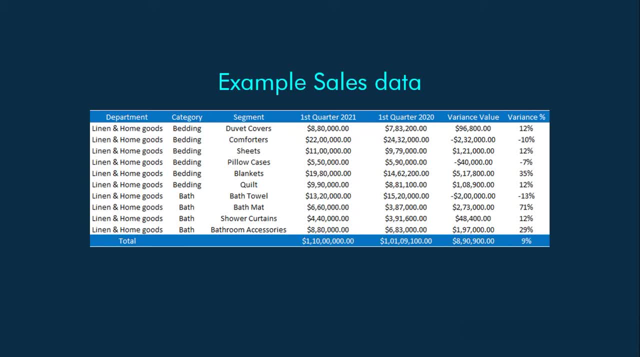 an example, nothing to do with any of the company's figures or whatever, Just in a sample data which I like to have it on this video for an analyzation. It's a raw data and let's see like what are the informations we can take it from this sales information. Let's. 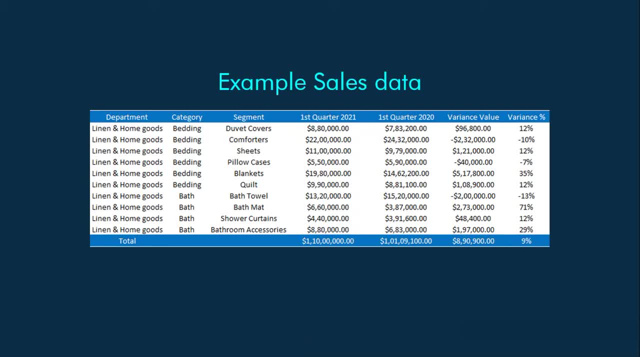 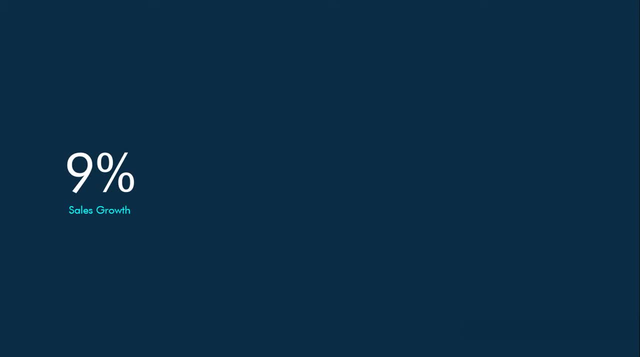 see from the raw data what we have seen it now. This is a image from the $100 website. From the data we have been able to see that the Chile department has creating more products. thus far has a sales increase of number of 9% compared to last year's first quarter. 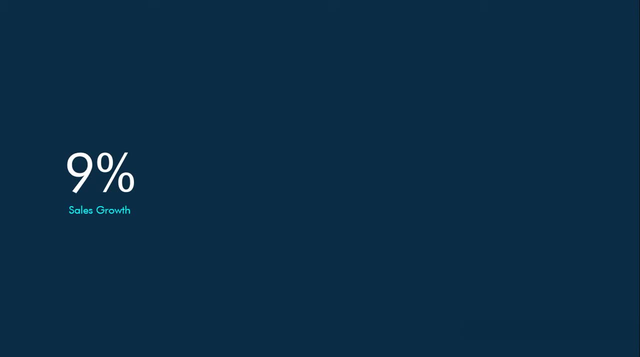 That's good. actually. The department has increased the sales increase by about 9% Number of good, but is it really doing good? so to figure out those, we need to go in a further detail here. it will shows an idea. within the department we had two categories. 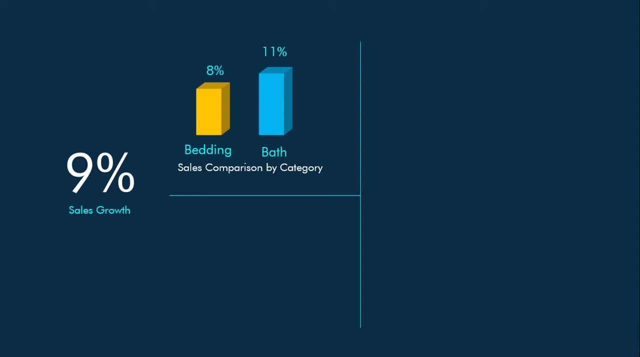 bedding and both. if you look at bedding category, it increased only 8%, whereas your whole linen and home goods department has a sales increase of 9%. whereas the bedding category has increased only 8%, which is lesser than your overall department sales increase. so it shows that there is an issue with 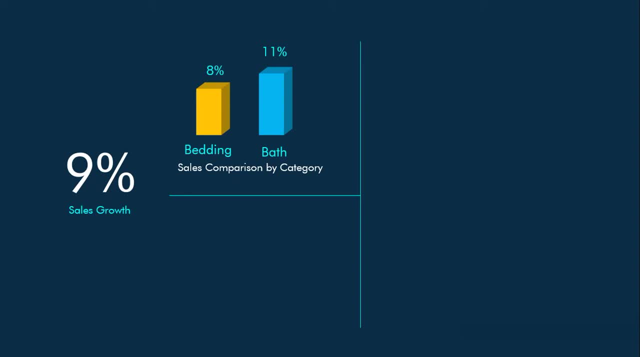 a bedding category. so we need to pay an attention to that category to fix it and then the both category looks good. but we need to go in a further detail here for a both the categories to know exactly whether the numbers are good or no, before I go in a further detail. the reason I told you the bedding category: 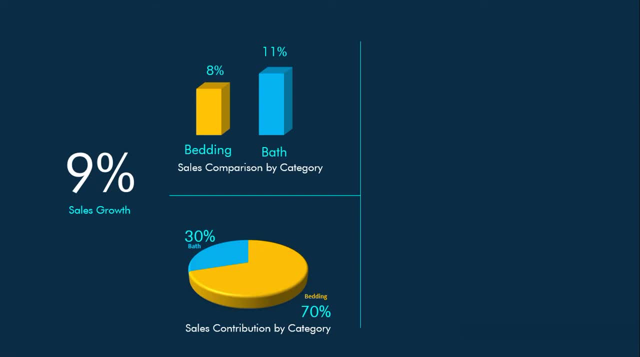 needs an immediate attention because, as per the sample data, what I shared with you in the last slide- the bedding category has a 70% of the sales contribution to the total department. imagine if a category has a 70% of the sales contribution to a total department which is has a less sales. 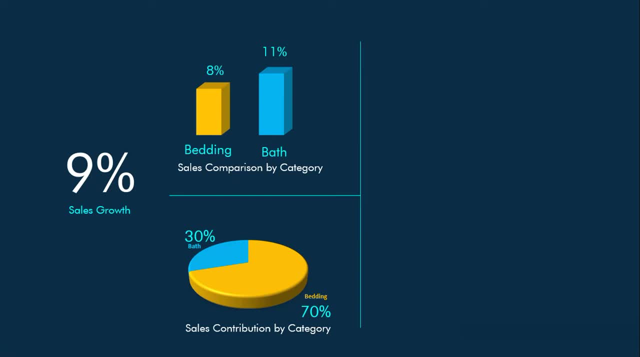 increase than your overall department sales increase, then there is an issue which we need to address it immediately to fix it. the next thing we I like to show you like we have a the sales increase percentage and then the sales growth information on a category level. but we should not stop it over here. I like to take it again in a segment level. 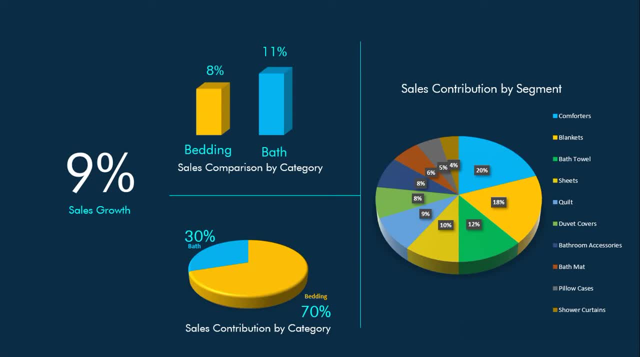 before I check my segment level, the sales variance, we like to see the sales contribution by segment. why we need to say this? because you you can see over here from the raw data what we have seen it in the last slide. we put a sales contribution by segment. out of those 11 segments, only three segments contribute. 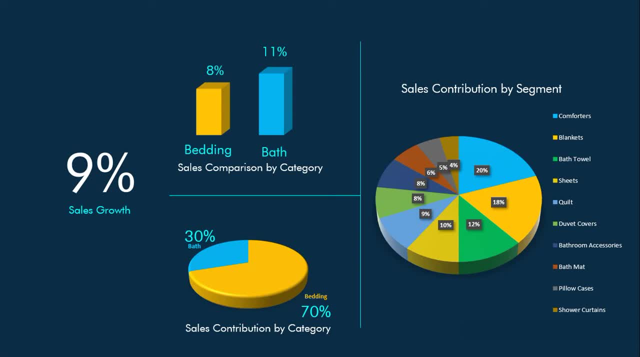 about 60% of your total department sales. what it indicates? it indicates if we have a better focus on at these three segments and if we do a special care on those three segments when we do assortment or when we choose a product or the range plan or the having a supplier. 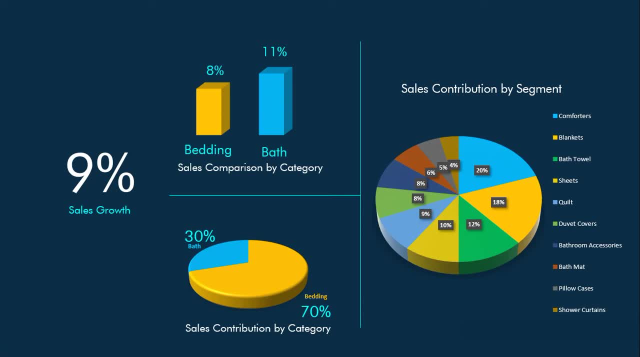 and role up unit area and then the contrary and when you fit it to, the department sales fall under these three sections. we can secure about 60% of our pickup sales. if we can have right focus over these three segments we can secure about 60% of our department sales. let's go into 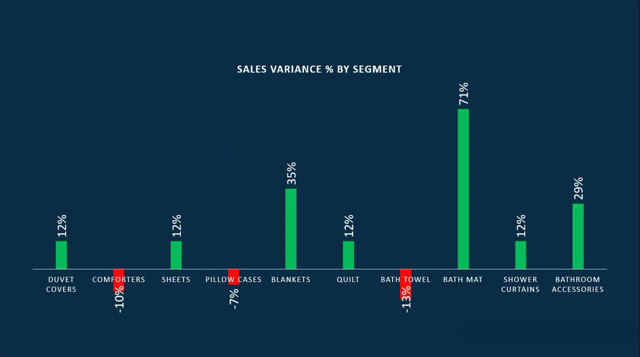 further detail, as I told you like we need to see the sales variance percentage by segment level. this is a chart which shows doing and what are the segments. we have an issue. it's very clear that the comforters- comforters- has a sales drop of 10 percent, which is higher than the total department sales increase percentage. 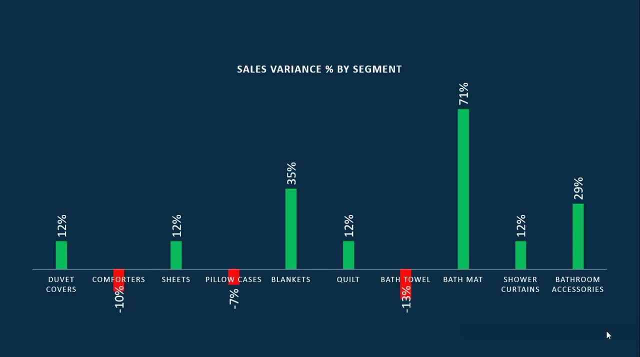 because we have increased, the total department has a good has increase of nine percent, whereas the category- the comforter- fall under the category of bidding. the category has a sales increase of eight percent, whereas the comforter sales drop is 10 percent, which is really alarming. we need to. 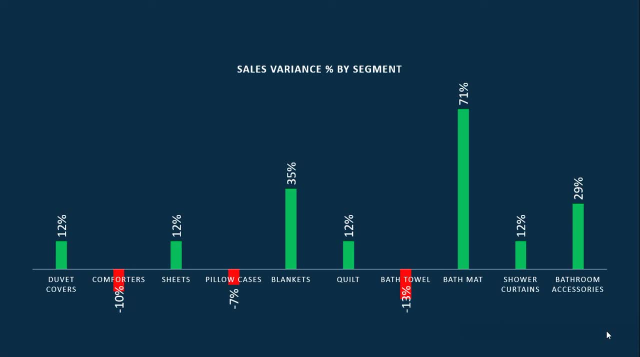 have immediate attention over there to fix it. if not, then in the coming quarters the overall, the total department, will be in a negative. we lose whatever we gain it in the first quarter, we will lose it in the second and third quarters if we don't fix it. the reason i'm saying this: if you 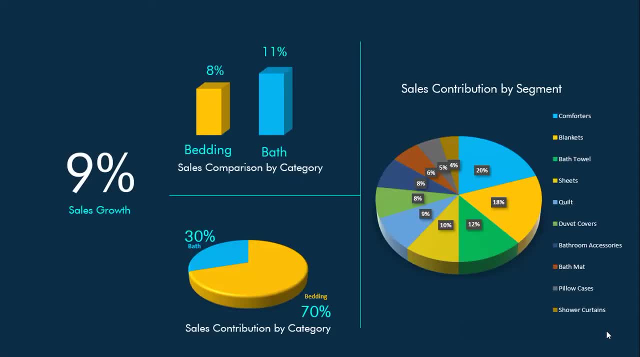 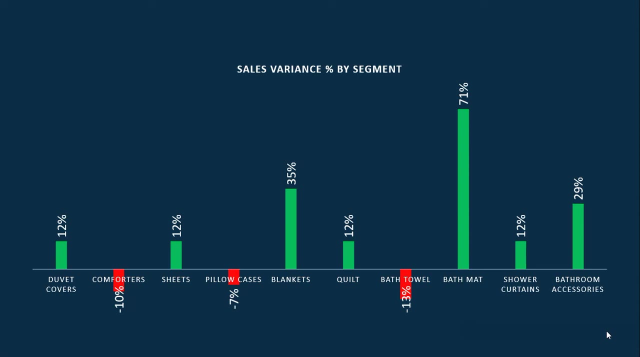 look at the segments. segments contribution uh to the department. comforters are the highest contributing segment in the department. if a segment has highest contribution to the department which is falling about 10 percent, then which clearly says that we are in trouble. so someone has to address that issue and then it has to be fixed on a priority basis. 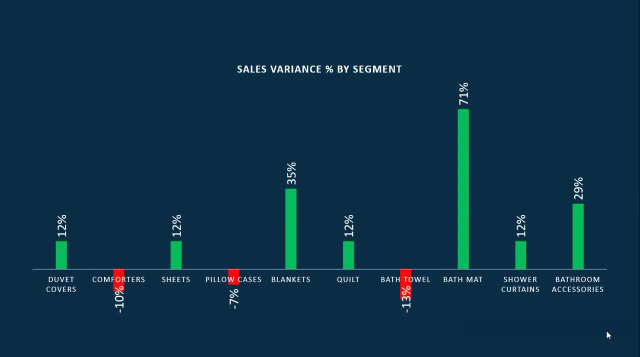 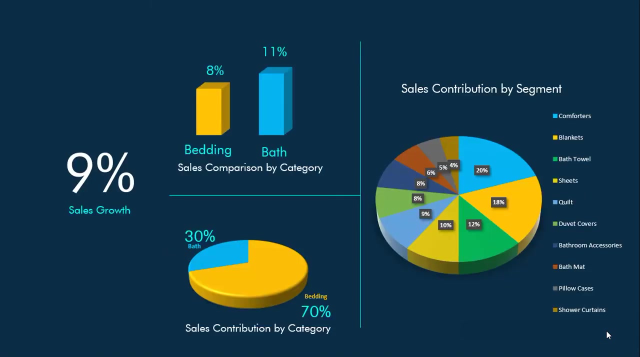 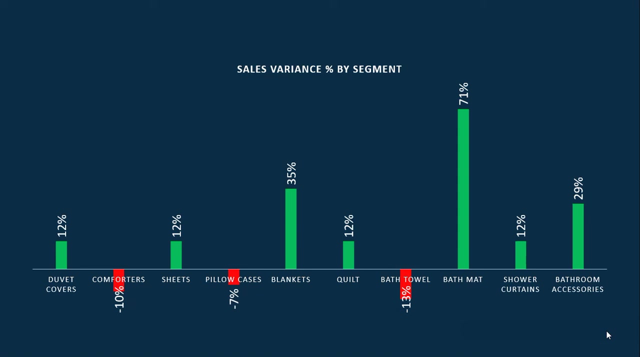 to recover the completion of the department and then we have to fix it on a priority basis. incident two: we are at the third segment and it's the second segment. the company has хаodesd uh right k easy um that out of top three segments, which contribute 60% of the total department sales. 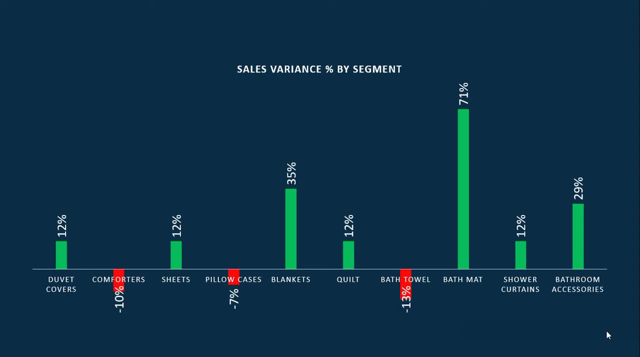 out of three, two are an issue: The comforters and then the baths travel. These two segments are negative And if the same trend continues, then in the second and third quarter the overall department will be in negative figures. How we need to fix this. 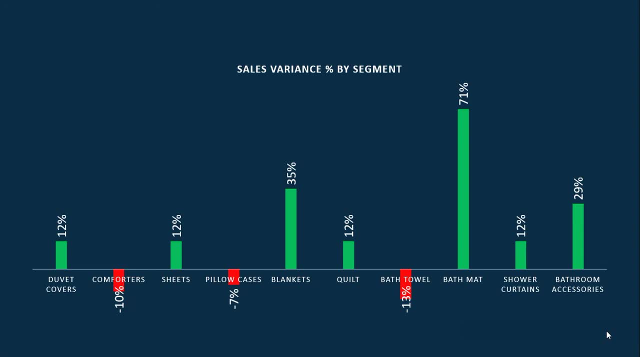 So what we have seen it now. We have seen it in a category level. After that we started analyzing by segment level And then we noticed that out of our top three segments, two are having issue. So what we need to do now: 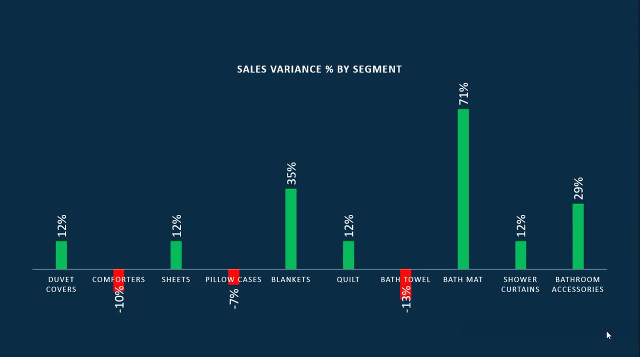 We need to go by supplier And then we need to go by product level if needed. What are the things we need to address? We need to check: is there any supplier issue or the supply issue, And then we need to check the availability of those items. 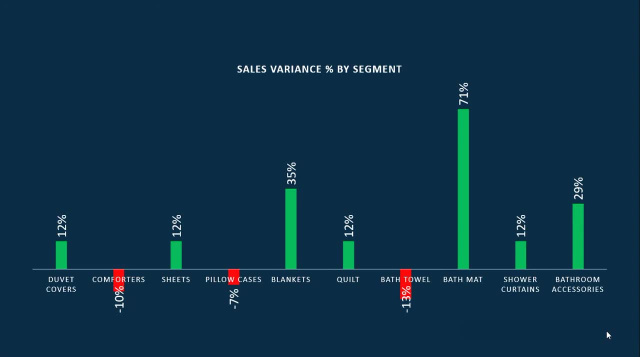 Or the assortment or the- whatever the top selling excuse we have it in these segments, We need to check those availabilities. And then we need to visit the stores to check the store presentation of these segments. And after you do this all, after you do all this analyzation, 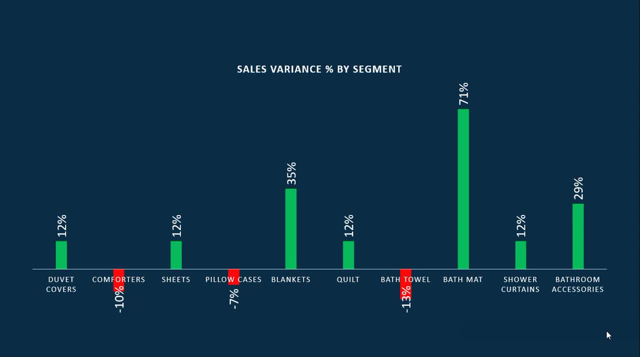 if you think there is no supplier issue. if you think there is no supply issue, there is no assortment issue. Even the store Presentation is good. If you're still dropping, then there is one more message the numbers are giving us. This is a time for you to refresh your assortment.